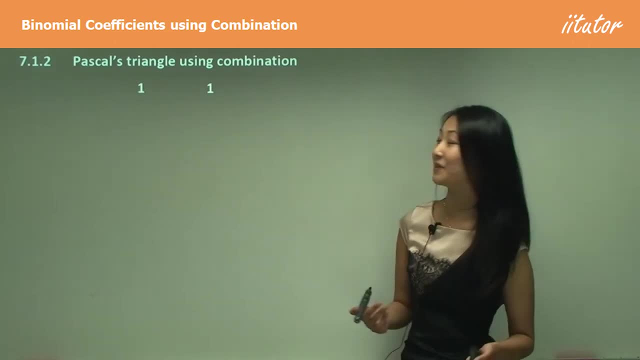 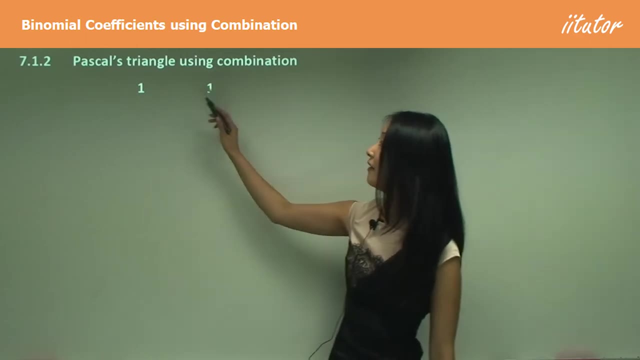 find these numbers. So we know that Pascal's triangle starts off with one one, and we can actually use combinations to work out these numbers. So one and one can be worked out by having one C Zero and one C1.. So let's just practice putting that into your calculators, So you just need to. 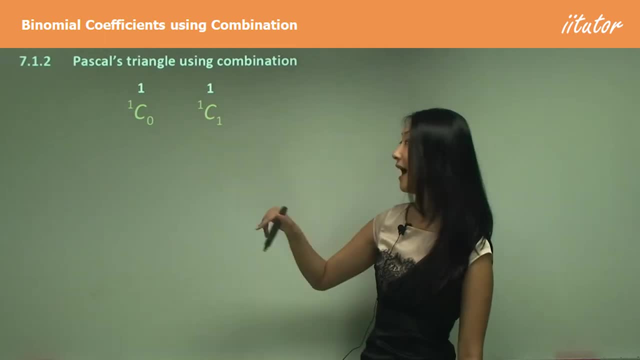 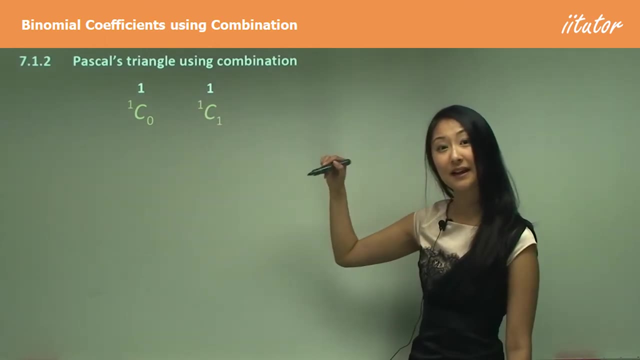 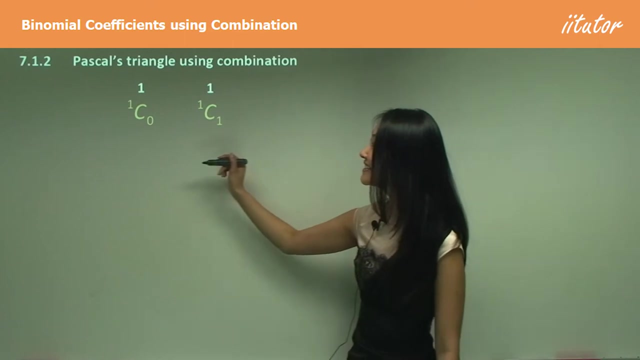 press one and you'll have a little C button. So shift that and zero And do you get one? Good, Great. Now let's practice with this one. So put in one C1 in your calculator And you get one as well, don't you? Exactly. So you can see how we use this combination to get one and one. But how do? 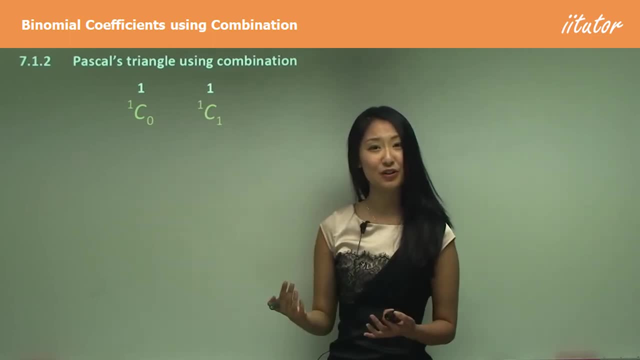 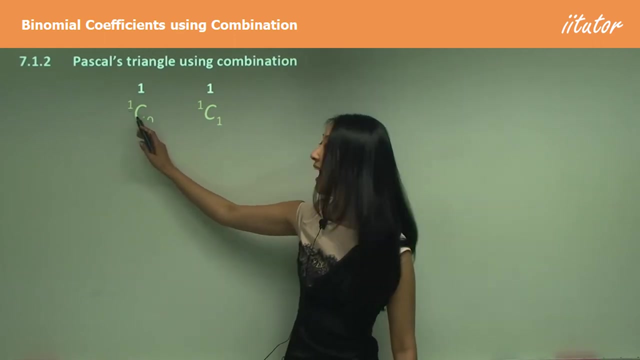 we know What combination to put in. So this is what I'm going to try and show you. There's a pattern to that For one and one. you know that this is the numbers that's used as the coefficients for the index of one. So that's how we start off with the number one, there And here we always start off. 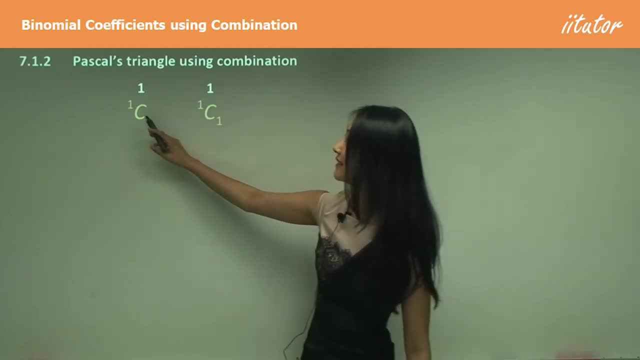 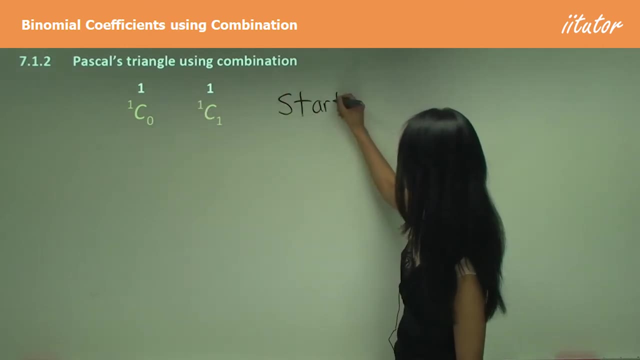 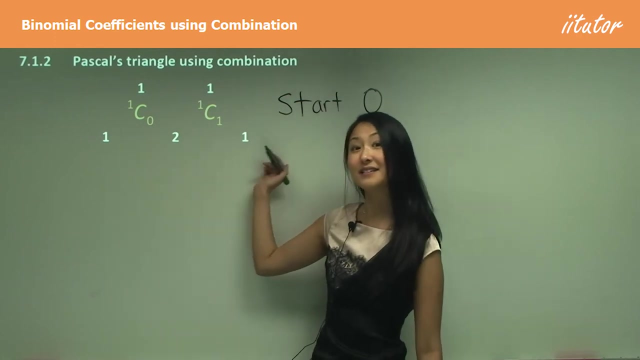 with zero, So it's actually quite simple. So this is what the index of this is used for, And that we always start with zero. Okay, Now let's see how it works for the next line, which is one, two one, So we can use the. 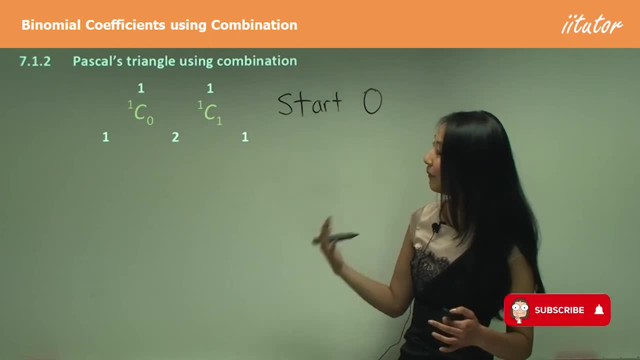 combinations again to get these numbers. So how we know what combination to use, remember how I said. well, this one was used for the index of one And this is used for the coefficients for when we're expanding, for the index of two right. So that's how we know We're going to start off with two up. 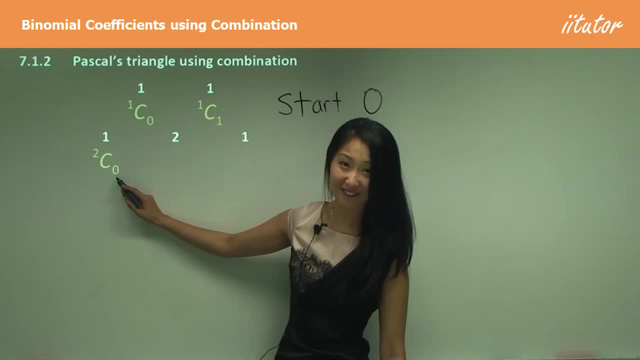 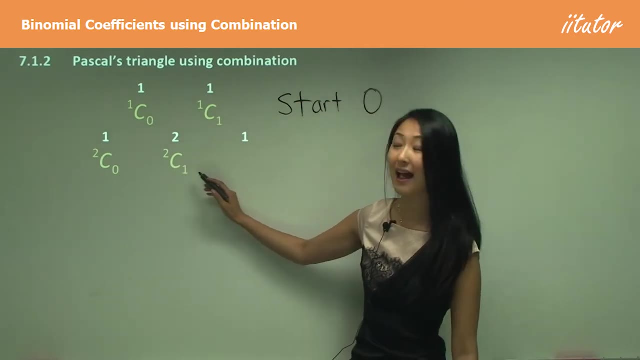 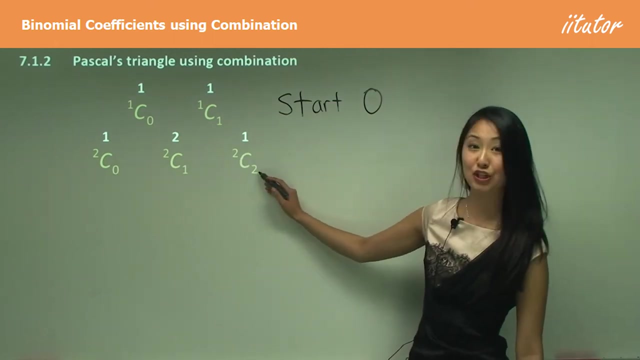 here and remember: this always starts off with zero and the next one is just going to be 2c, and this you just plus one, so it becomes one. finally, that becomes 2c2 there and the last one here. these two numbers should always be the same so we can have a quick check. does this give us? 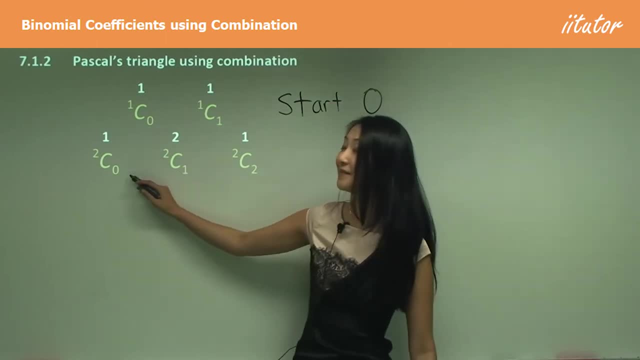 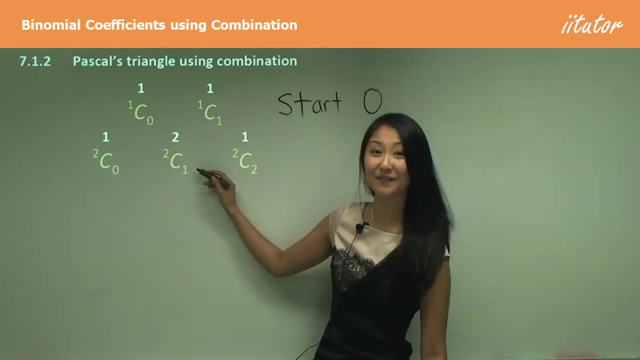 those numbers. so let's just check this one, okay, so put that in your calculator. so remember two and then c and zero, and you should get one. what about this? one, two and then c and one. good, it gives you two, right. so you can see, this is how we can use combination to work out these numbers. 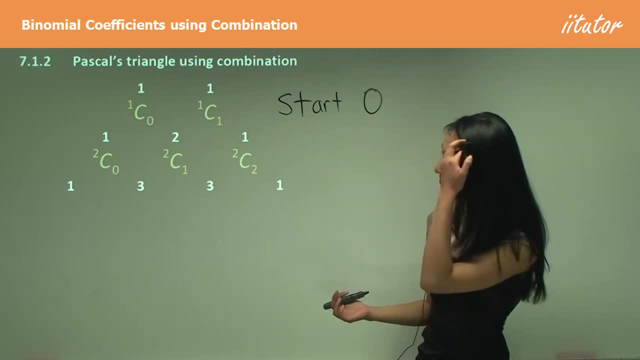 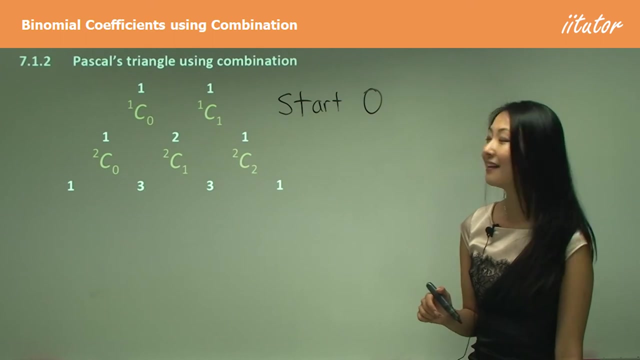 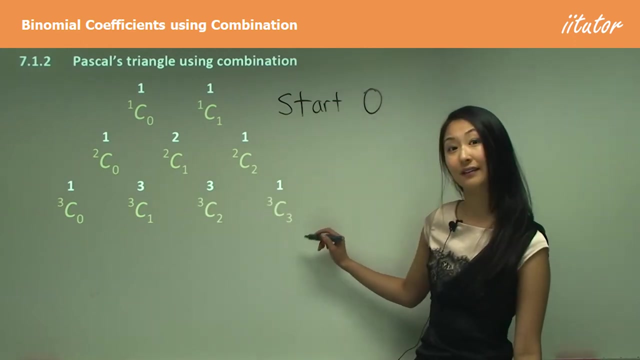 all right, let's have a bit more practice with the next line. so here we have 1, 3, 3, 1, and to get these numbers we're going to use this formula for combinations. so this is used for the index of 3, So we're going to start off with good 3C0.. And this will be 3C1, 2,, 3C3.. And if you put this: 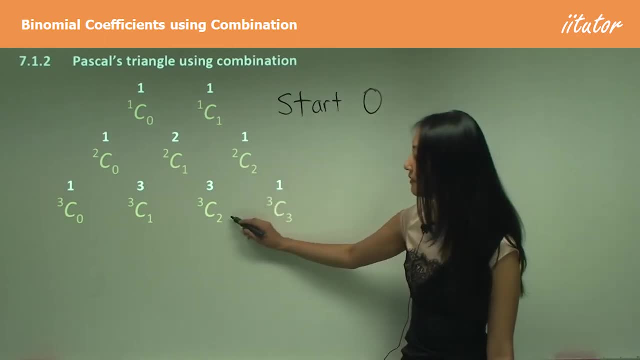 number in your calculator, you're going to get 1.. And if you put this, you get 3.. And this gives you that 3, and this gives you 1.. So this, these combinations, is going to give you these four. 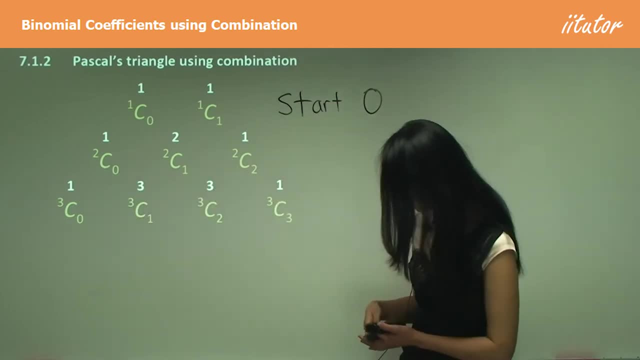 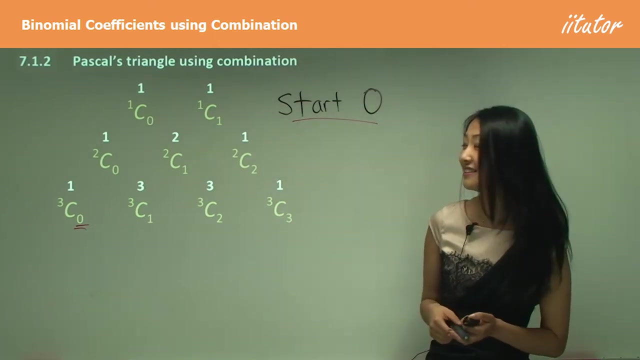 numbers essentially All right, Okay, And you can kind of see that although this is the first term, it's always starting off with zero there. So just remember that we're starting with zero, even though we call it technically the first term. Let's try and use combination to get the. 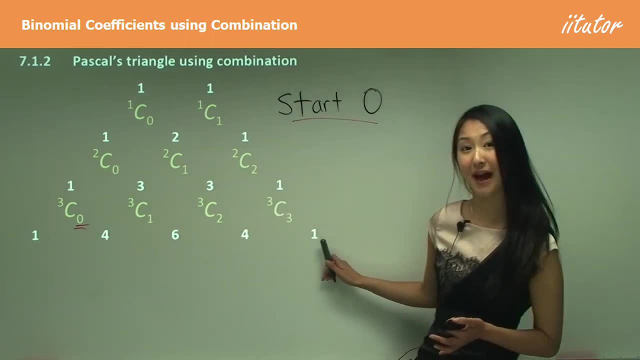 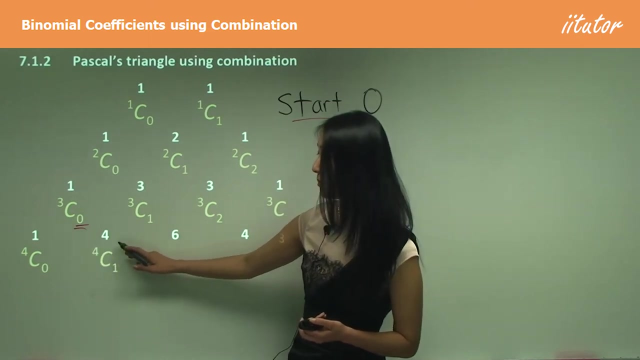 same numbers as we would by just writing out the Pascal's triangle for that. So we know that because this is used for the index of four, right, That means we're going to start with 4C0 as our first term And then 4C1 will be our second term. Add another one, C2, become our third. 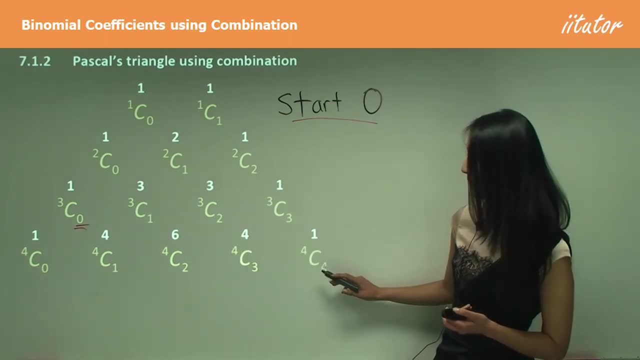 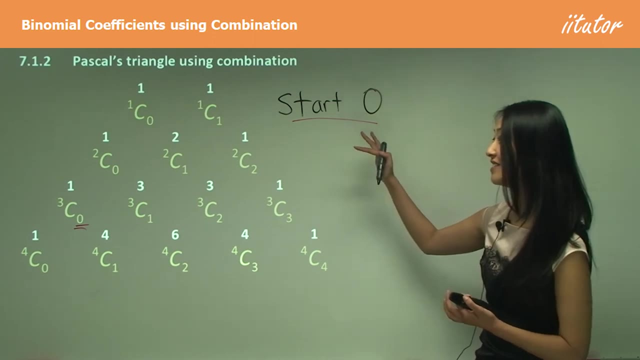 term, 4C3, our fourth term, And finally 4C4 as our fifth term. So this is how we use combination to work out these numbers without writing it all out. Why this becomes useful is if you have power of 20,, for example, it's going to take you a really long time to go down and get the. number right. So if you have a power of 20,, for example, it's going to take you a really long time to go down and get the number right. So if you have a power of 20,, for example, it's going to take 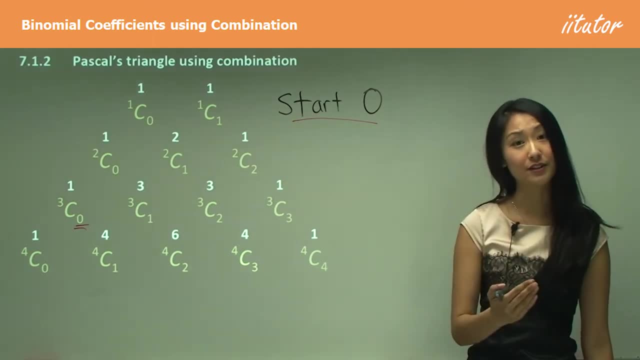 you a really long time to go down and write it all out, But it's going to be a lot easier to know that the first term so that is always going to be 20C0, right, And the next one's going to be: 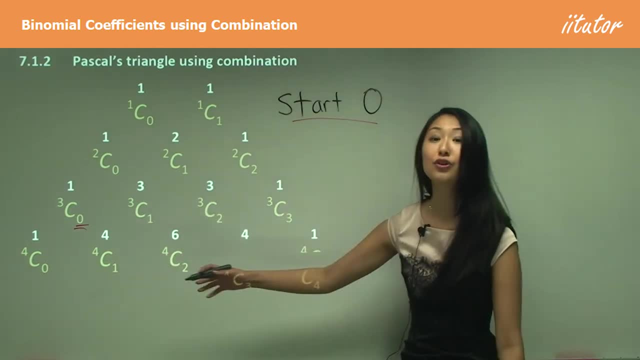 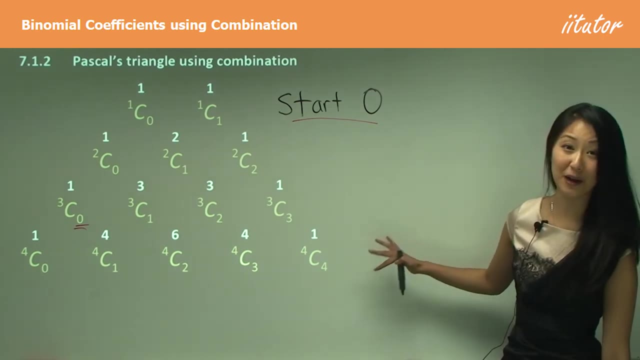 20C1.. The next one, 20C2.. So on until 20C20.. So can you see how this is how we use combinations. So that's the first point I want to make is how to use combinations instead of drawing.